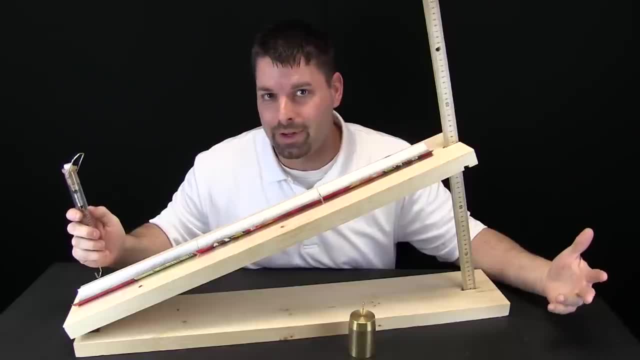 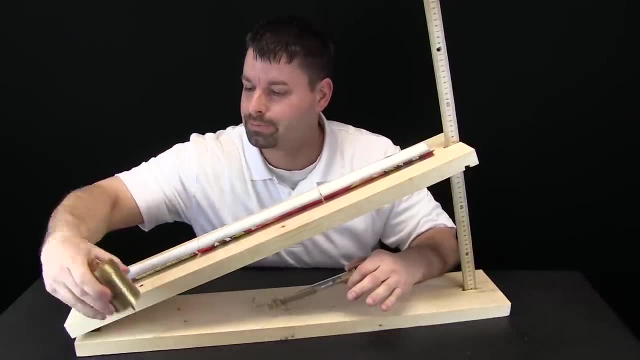 take a closer look and see what will happen. What do you think will happen If our work is made easier? what kind of reading will we get on our spring scale? So let us find out what happens, Let us put our weight at the bottom of. 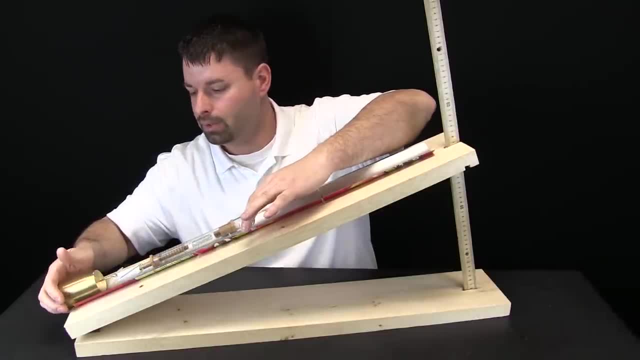 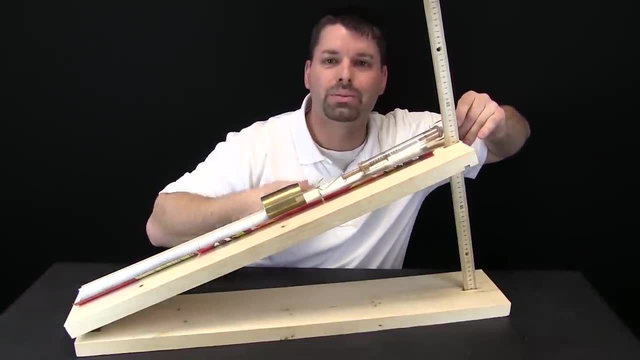 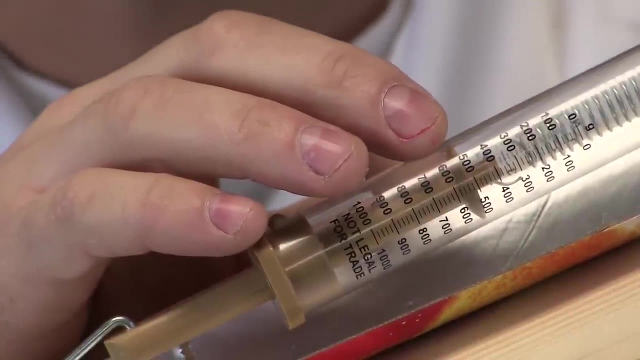 our inclined plane. attach our spring scale and now let us move our weight. Moving the weight, we are going to zoom in and take a look at what our spring scale says. Take a look at our spring scale. It says it is taking 500 grams to move this. 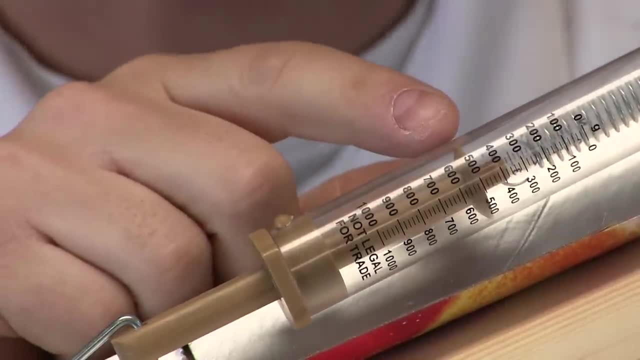 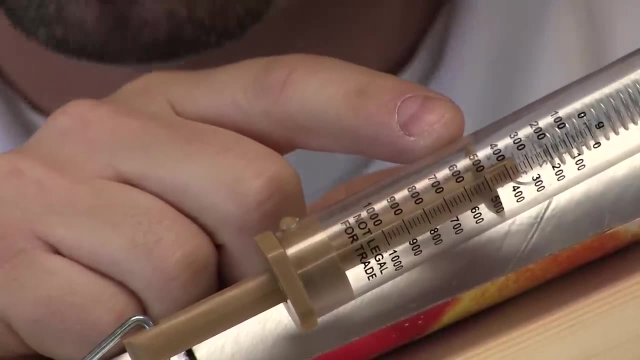 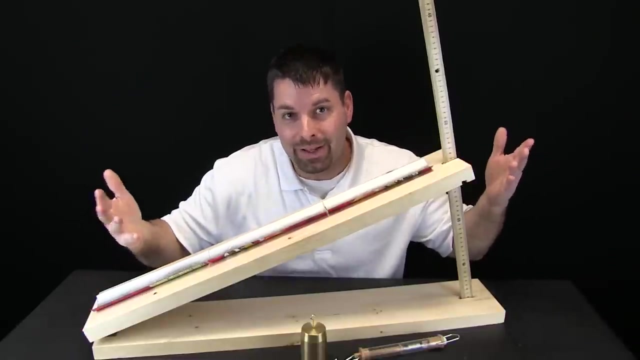 weight. Remember when we lifted the weight straight up, it took 1000 grams. Now, using our inclined plane, it is taking 500 grams. What does that mean? That means that this inclined plane has made our work easier. So what do you think will happen when we change the angle of our inclined plane? 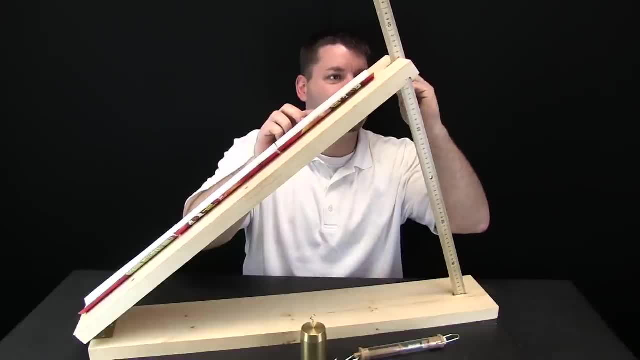 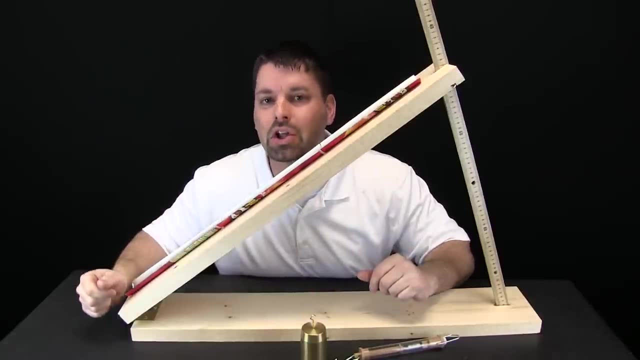 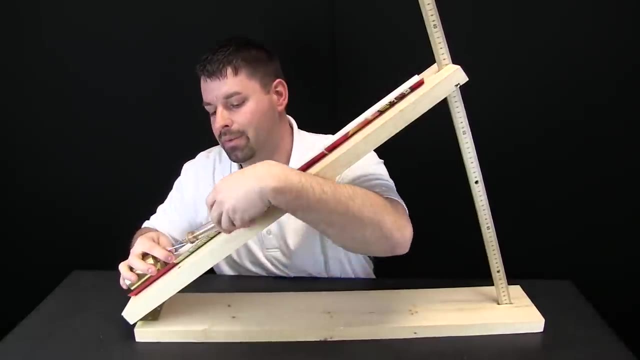 What happens if I take our inclined plane and take it up higher? What do you think will happen? Let us take a look. I have my weight, I have my spring scale. put the weight on the bottom of my inclined plane and now let us move the weight. 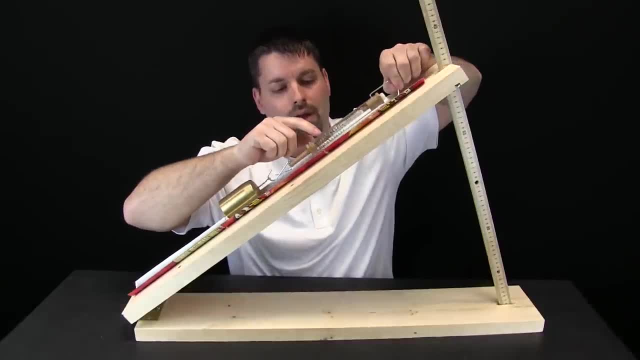 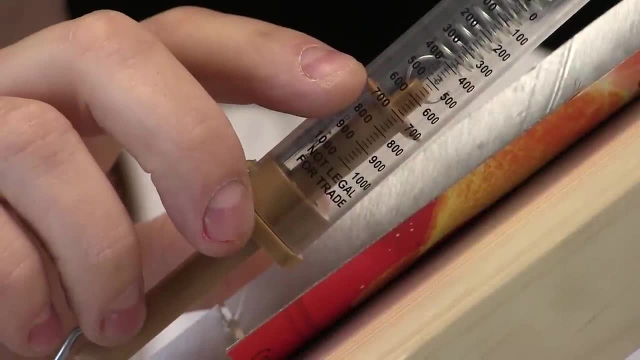 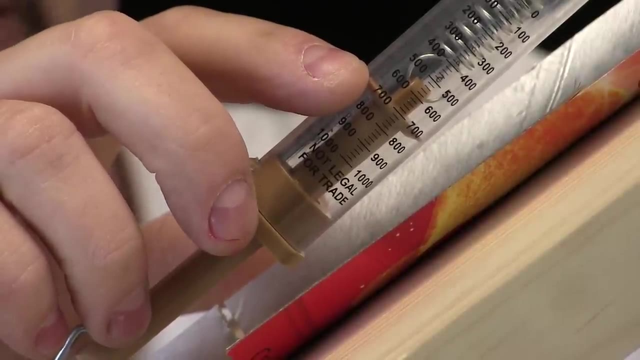 with our simple machine. We are going to zoom in so you can take a closer look at our spring scale. So take a look. Our spring scale is reading 700 grams. Remember, this is a 1000 gram weight. Our work is easier when we use the inclined plane, So let us think about 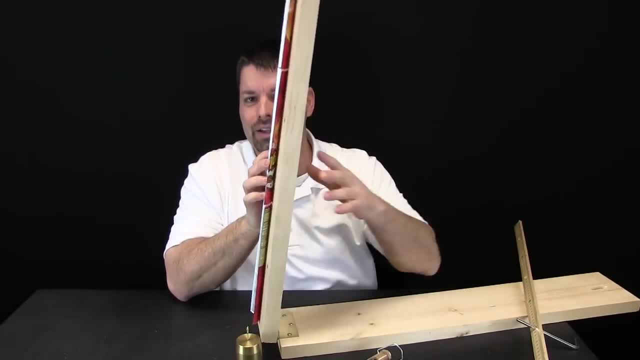 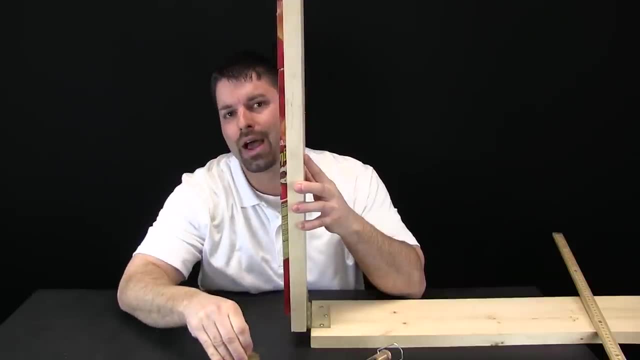 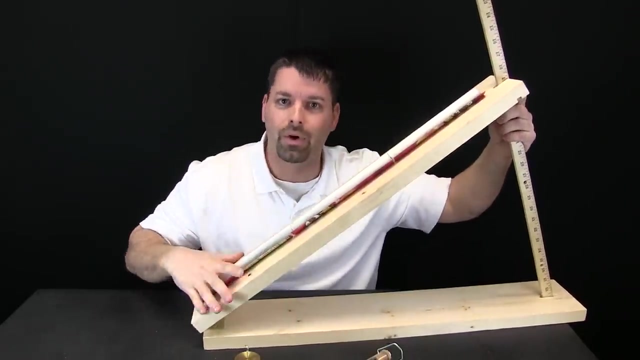 this inclined plane. If I were to take this inclined plane all the way up, well, that would just be like lifting my weight straight up. It would be a 1000 grams. But when I take my inclined plane and I angle it down, I am making my work easier. What would happen when I drop my 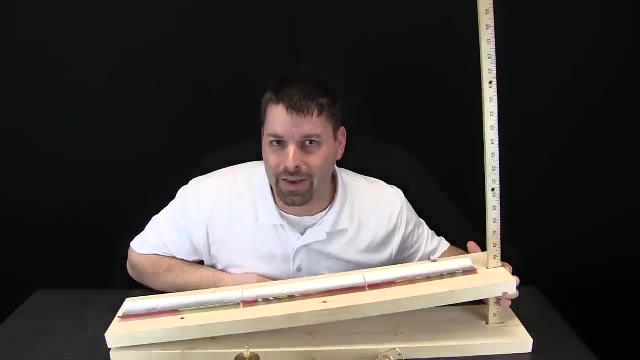 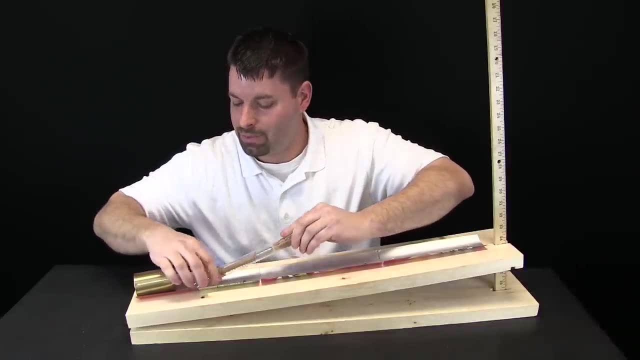 inclined plane down even lower. Let us take a look at that. We have our inclined plane lower. Let us load up the weight, attach it to the spring scale and see what kind of reading we get. Here we go, I pull it along and we will zoom in and take a. 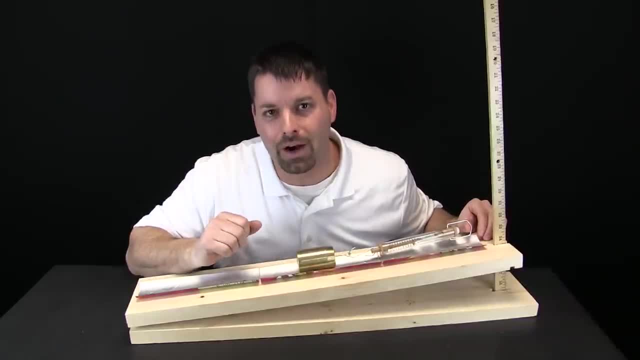 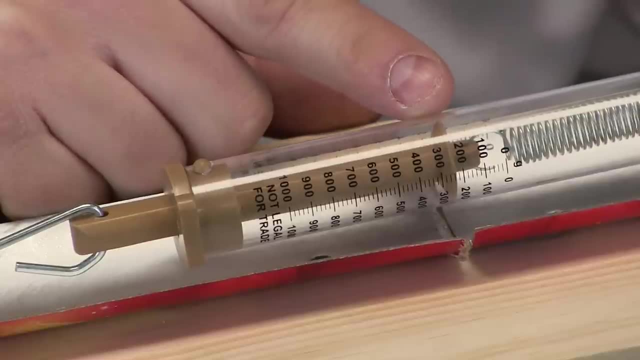 closer. look at the spring scale but you are going to see it has really made our work easier. This spring scale is reading 250 grams. Think about that. It is still a 1000 gram weight but it is taking 250 grams to move that weight. I would say our work has. 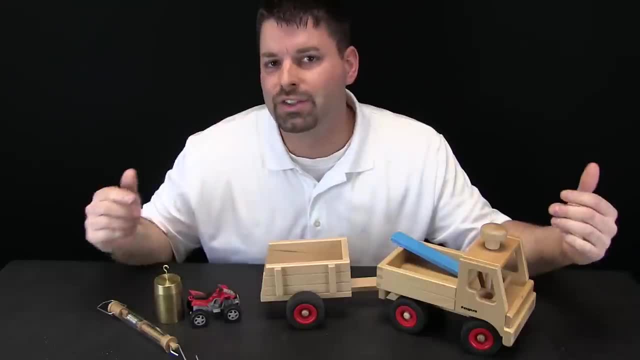 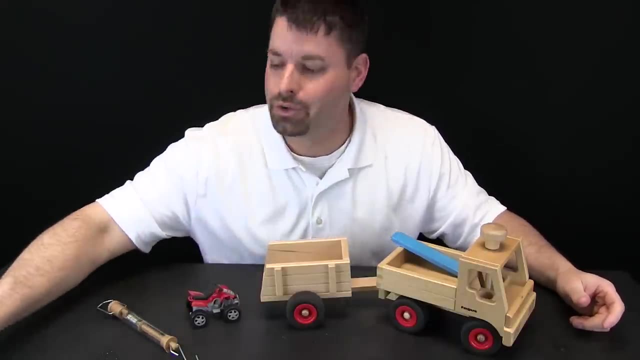 made a whole lot easier with this simple machine. So let us take another look of our simple machine, the inclined plane, in action. Instead of using this 1000 gram weight, I am going to use this four-wheeler, this quad. What if I had to load this? 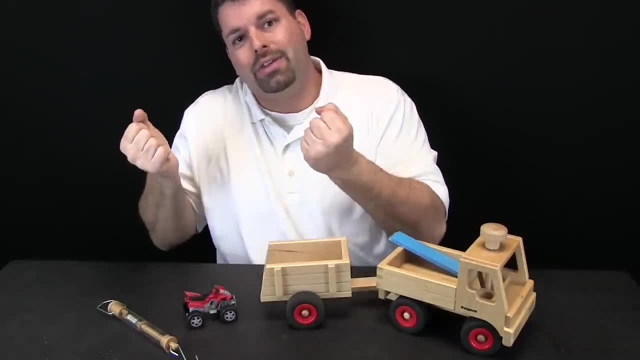 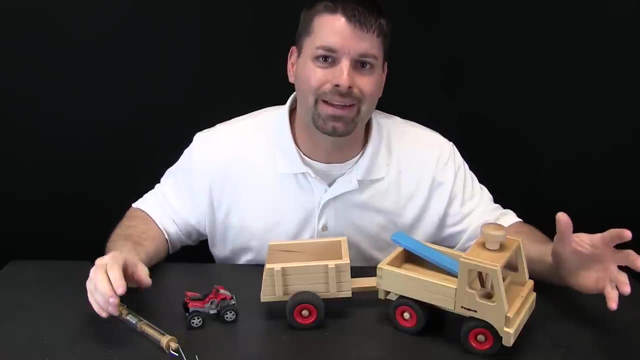 quad into the back of this trailer. Do you think I could actually lift that machine up and move it back into the trailer? I do not think I could, but I could use our simple machine, the incline plane, to make it a whole lot easier. So let us see if we can use some. 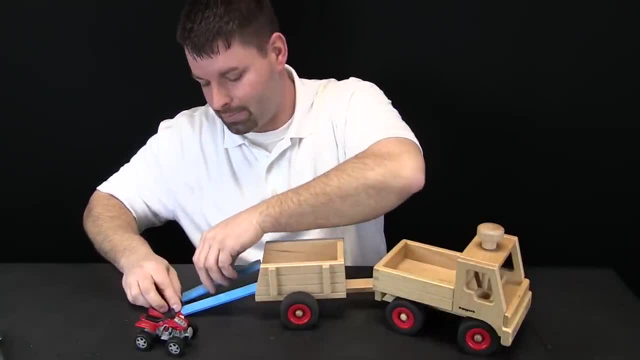 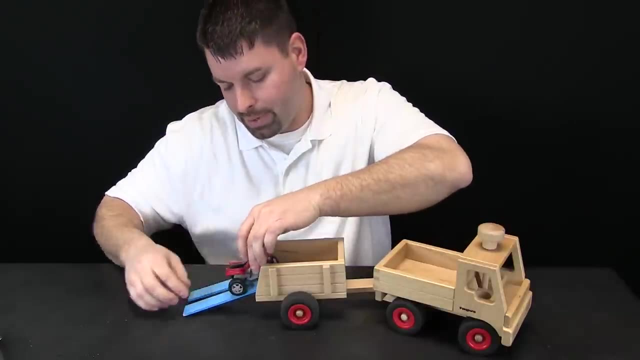 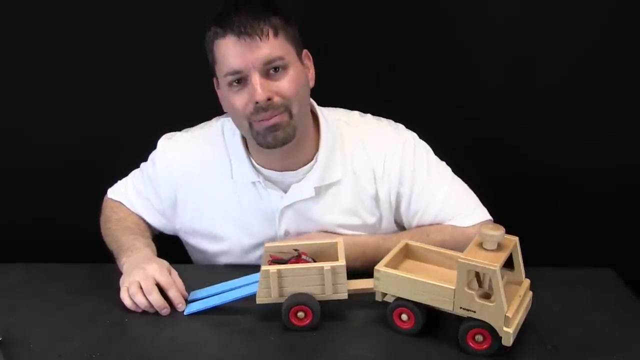 incline planes to help us load our four-wheeler. Put my incline planes up on my trailer and see if we can move our quad up the trailer instead of lifting it, and it works. That job was made a whole lot easier using incline planes. Now, incline planes may seem very. 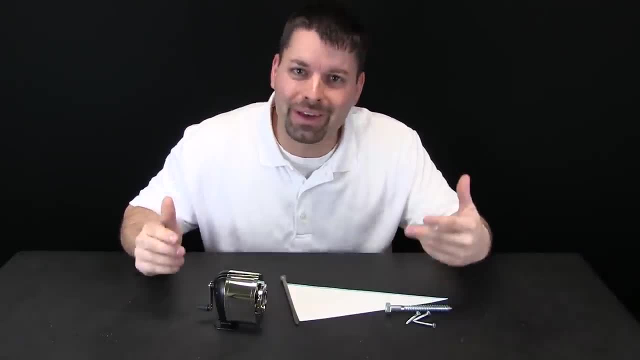 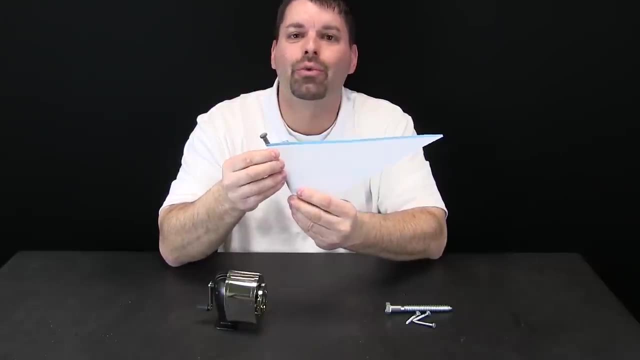 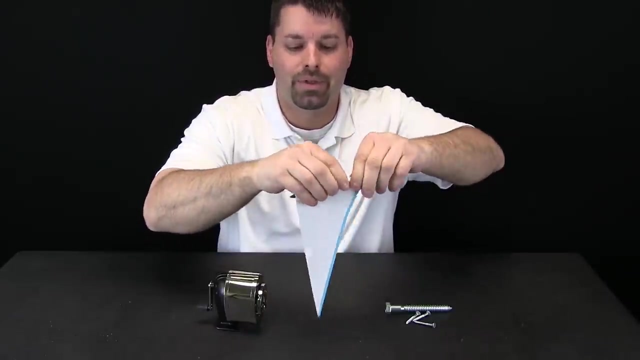 simple, but we can do really cool things with incline planes. Take a look at this. I have my incline plane, but watch what happens when I wrap that incline plane around something. Get it started. here I am going to wrap this and I want you to see what happens when I. 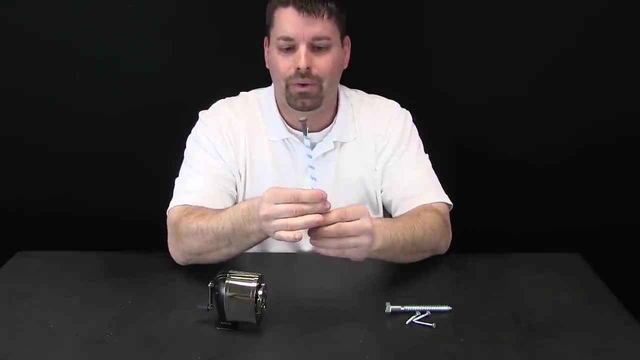 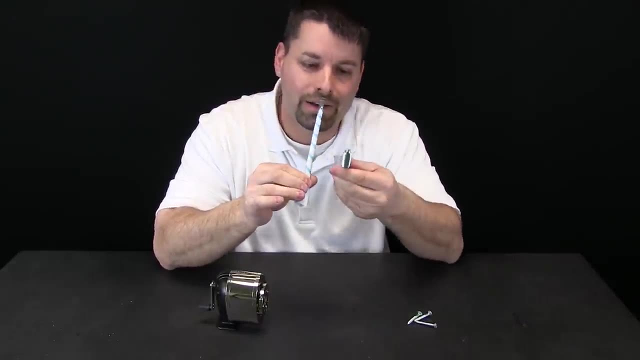 take that incline plane and wrap it up. What does it look like I am forming? Well, see the blue line at the top of my incline plane. It looks an awful lot like a screw. We have zoomed in so that you can see that. 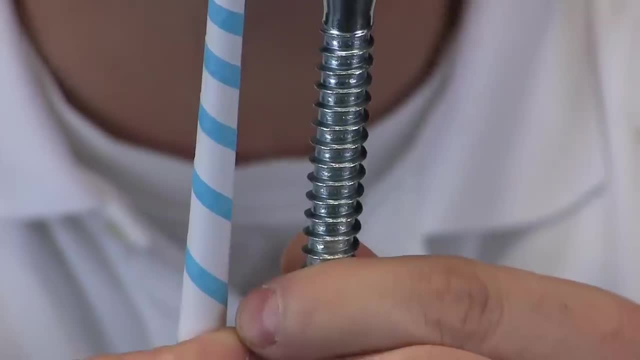 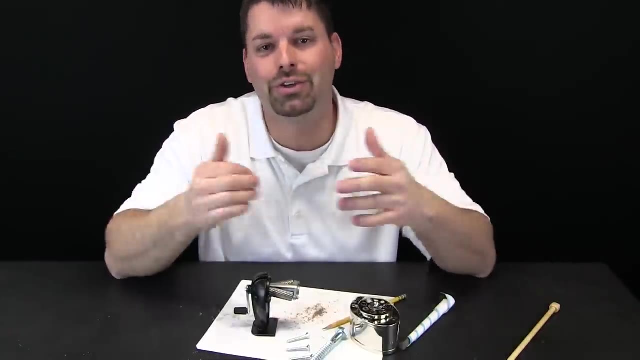 a screw is nothing more than an incline plane wrapped around a piece of metal. Incline planes and simple machines are all around us. See if you can find your own examples of simple machines anywhere. If you want to learn more about simple machines, check out. 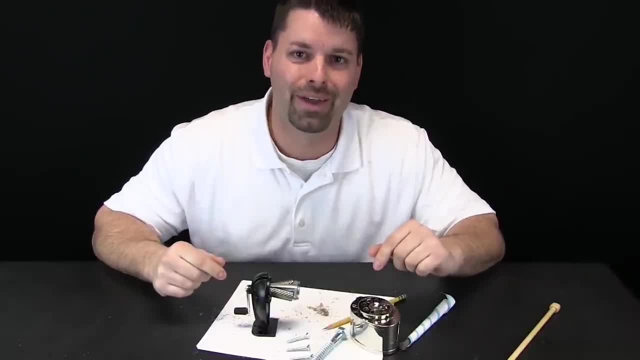 our links in the video description. Science is so cool, especially when it makes our work easier. Thanks for watching.